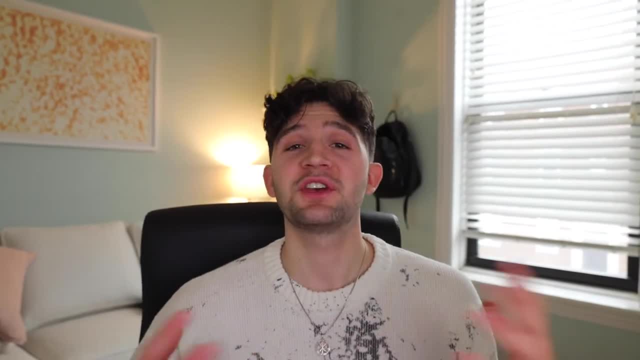 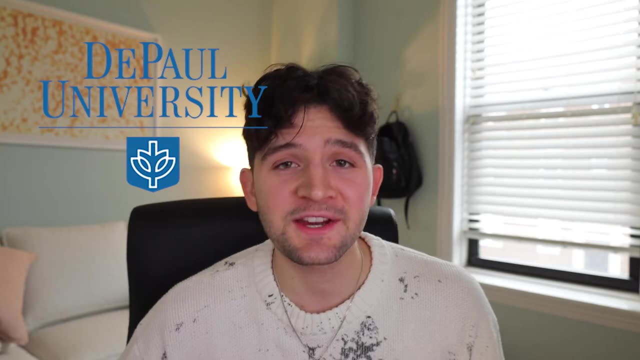 do the costs outweigh the value? My name is Sasha C. I'm actually a UX designer, So I am actually currently in the field of getting a master's at DePaul University in human computer interaction, And I want to tell you guys a little bit about what exactly it is, what to expect. 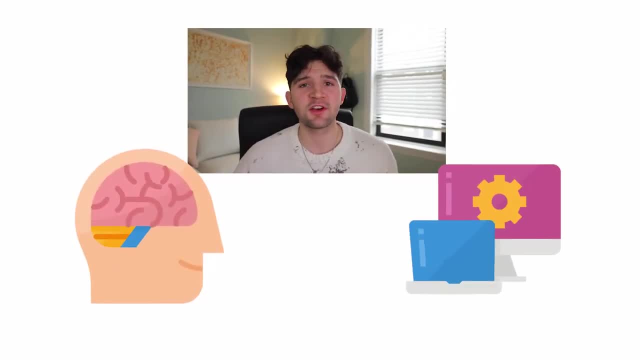 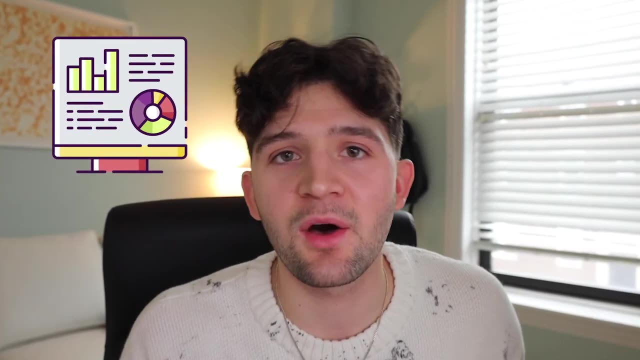 and if it's actually worth it. So people are fascinated, including myself, by the connection of computers and people. Now there are several different fields of study that are growing, dedicated to algorithms, and studies and research just based on ways on how technology can help. 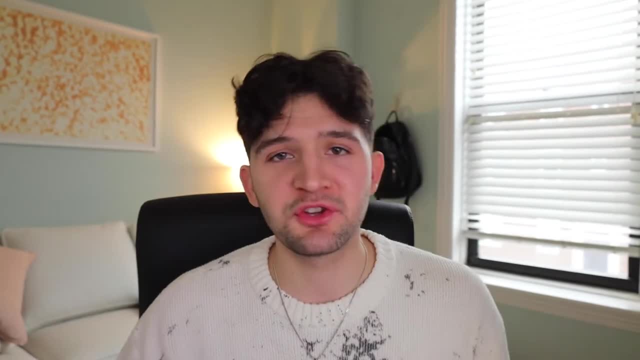 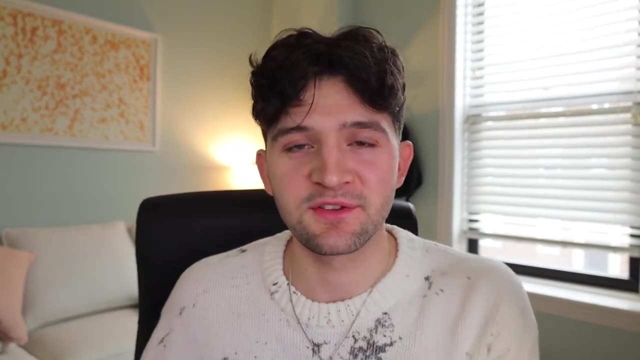 improve people's everyday lives. So what exactly is human computer interaction? What do these weird words even mean? So I'm actually just going to read a complete definition and then just kind of give my own definition. So human computer action is an area of study that involves better. 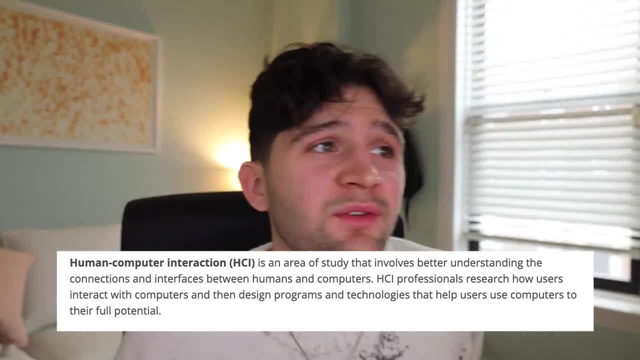 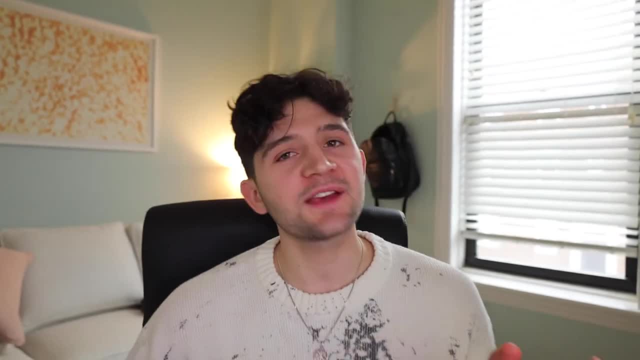 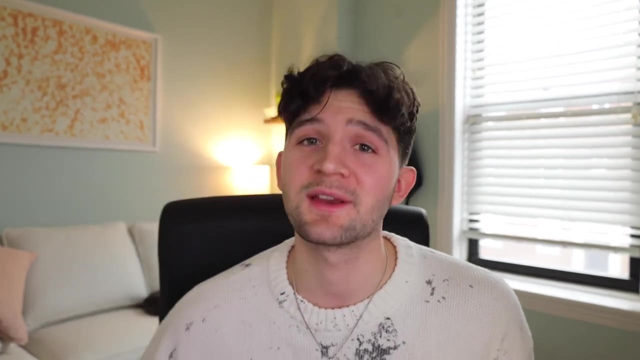 understanding. Okay, so now my description of what HCI is. So HCI is a really broad term And it's really just the development and research of ways you can improve people's lives through technology. That's the best way that I can really describe it. You have to like kind of understand. 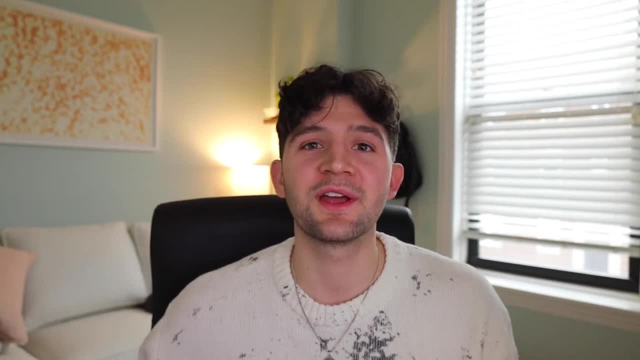 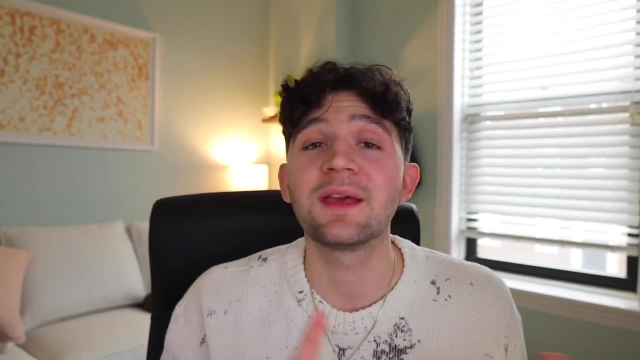 that you're incorporating so many different things. you're considering the user, the business, behind whatever you're making. So you have to understand what the goal is for whatever you're making. Are you trying to make money? Are you trying to educate? 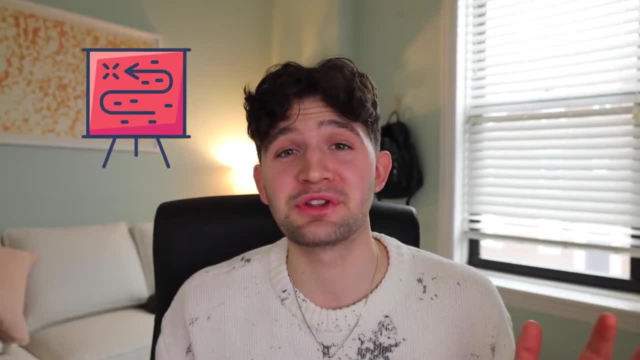 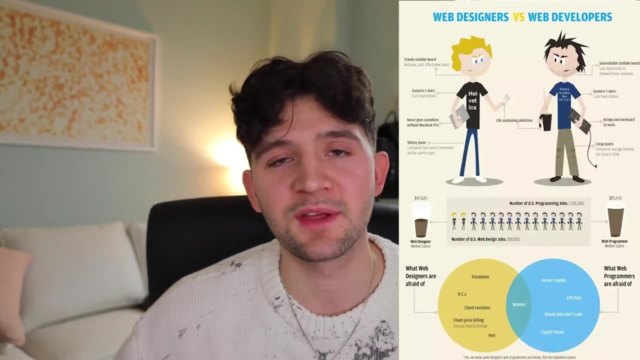 Are you trying to entertain And then you also have to work with what's actually functionally possible, such as like developers. if you're like putting together this prototype and you give it to a developer and they're like yo, I can't do this, it won't work. But there are so many different. 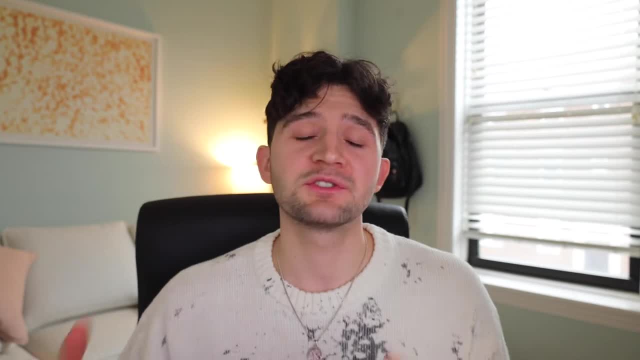 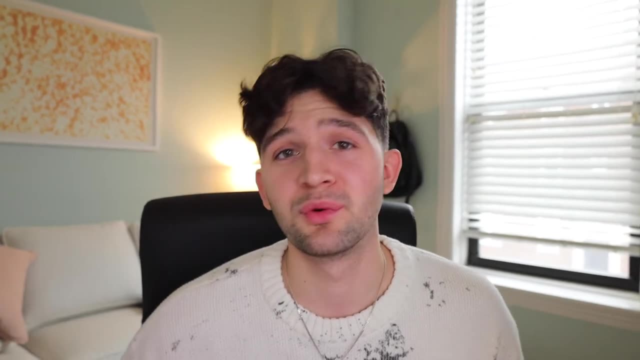 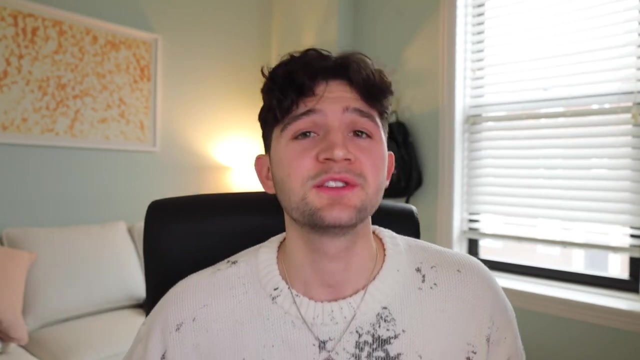 jobs in that field. It is kind of crazy. So specifically, just for example, I'm a UX designer. this is really just the idea that I design systems that improve either businesses or people's lives every single day. So, personally, a lot of the clients that I work with are actually business related. So a lot of the things that I'm 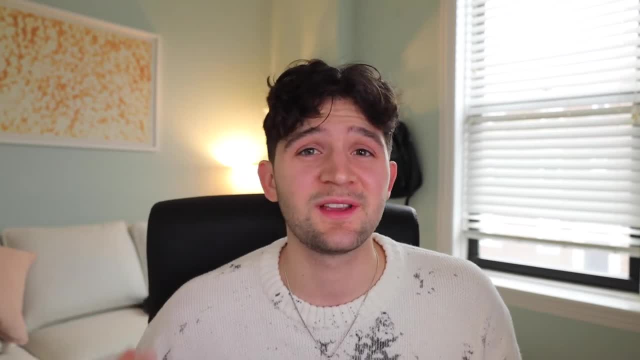 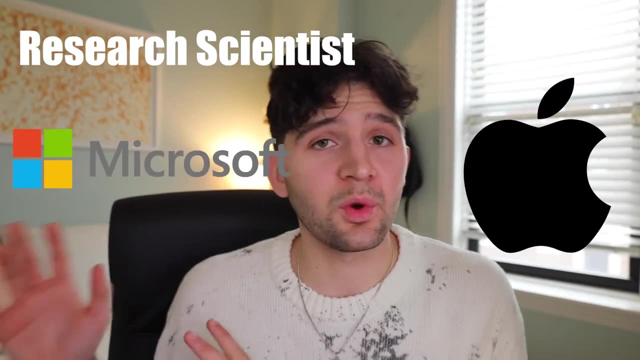 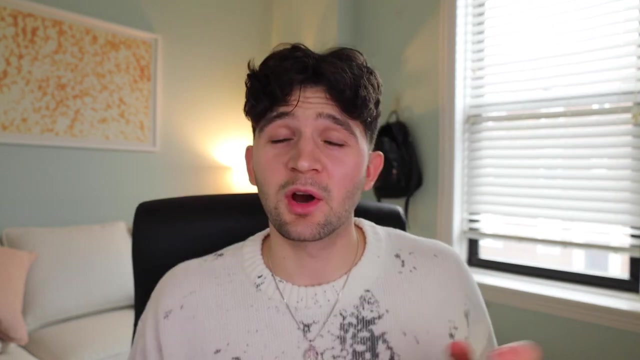 working on are technologies that can help improve business functions and business value. There are research scientists where literally like Apple or Microsoft will hire you to literally just do simple research on the process of how people are using their technology. And then there are product designers: they really focus on the process of how people are using their technology, And then there 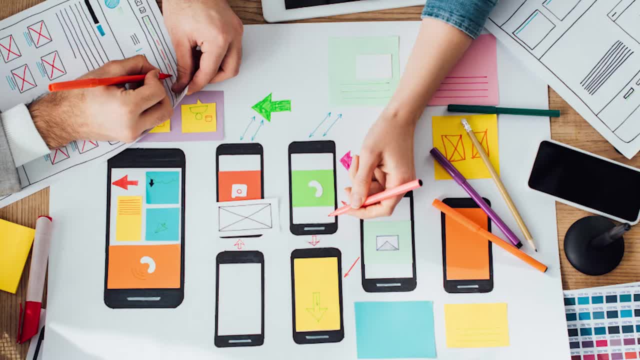 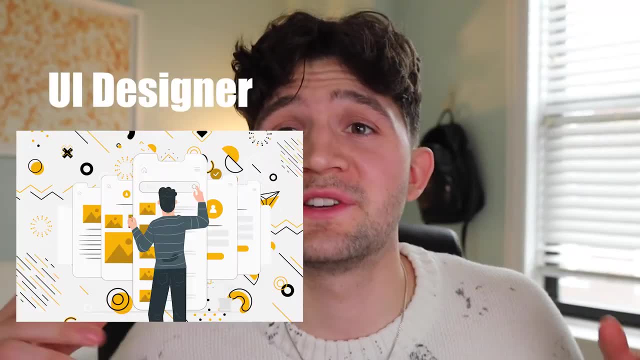 are product designers. they really focus on the process of how people are using their technology. on more visuals, I'd say they focus on, like UI elements, how people visually interact with interfaces online, And that goes into another role which you can do, which is UI design, which 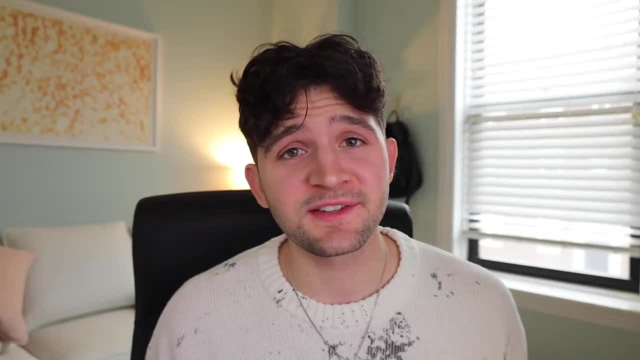 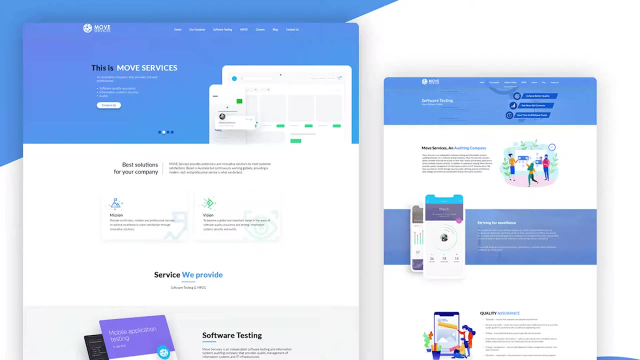 is literally just developing user interfaces, And a user interface is pretty much just anything that a user can interact with. So think of your iPhone screen: that's a user interface. or a website, that is also a user interface. there are information architects, And this is pretty much. 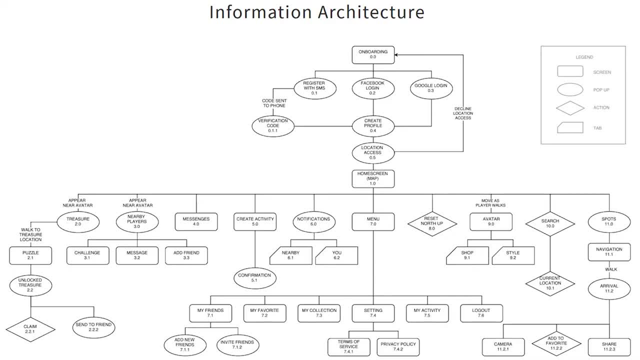 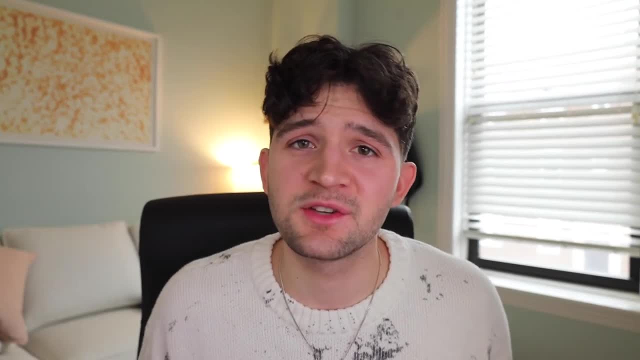 just the research of how a user can interact with a user interface. So there's a lot of research on how people are processing information when going through a design process, And I actually think this one can go past just technology. I've seen information architects work on things such as like: 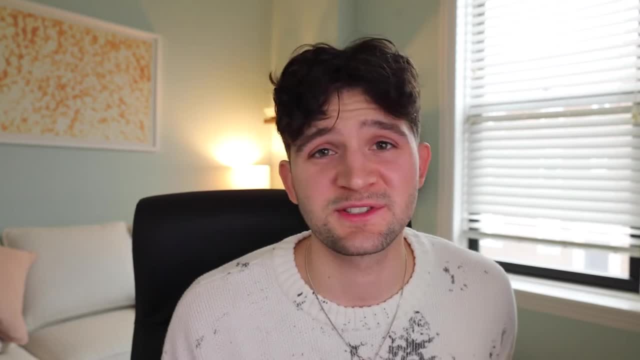 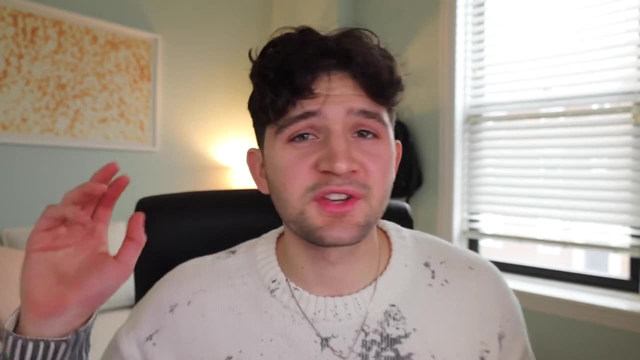 hospital systems where physical patients are actually going through a system And they're really researching the process that each patient is going through and developing a better system for it. And just to list off a couple more things, you can be a tech startup, a computer programmer. 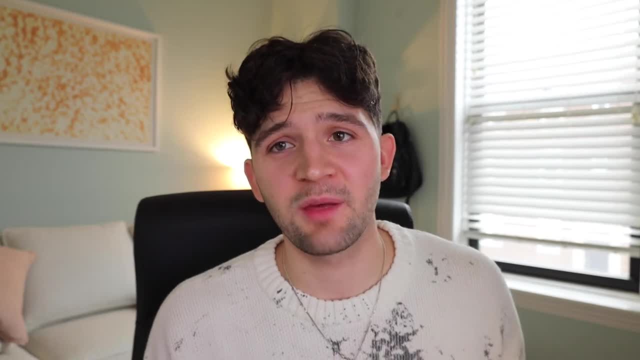 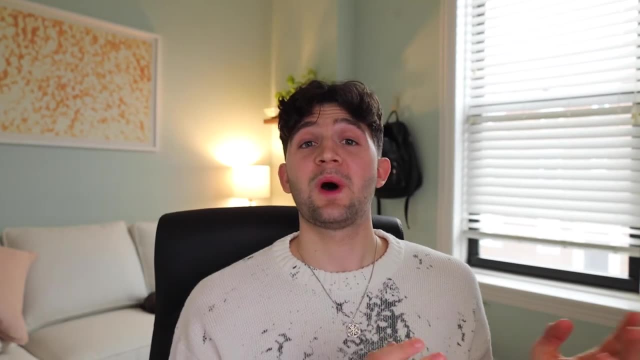 a systems engineer really a lot of front end development, And front end really means like the visuals and what the user is seeing. So getting back into the major a little bit and why exactly you would want to study human computer interaction other than just getting these jobs if 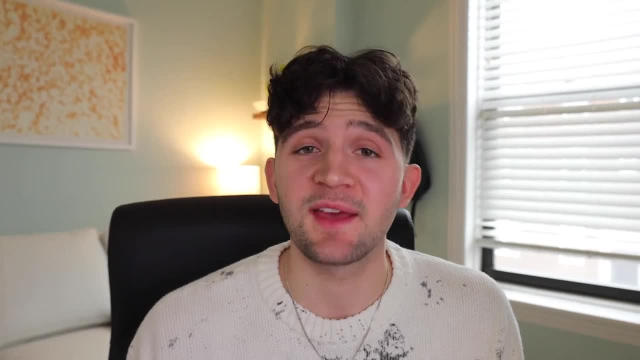 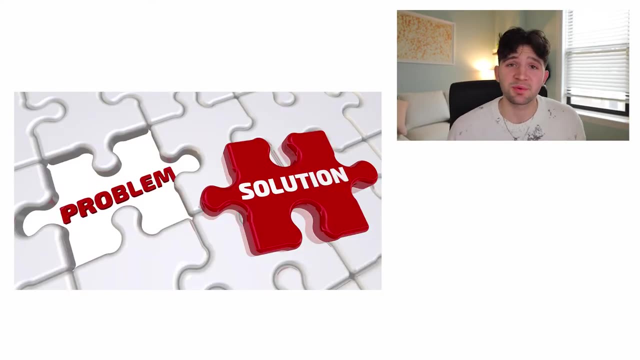 you're interested in any of these things, I'd probably say that, yeah, you should probably look into it and see if it's a right career path for you, If you're interested in solving super complex problems. you love working with other people. 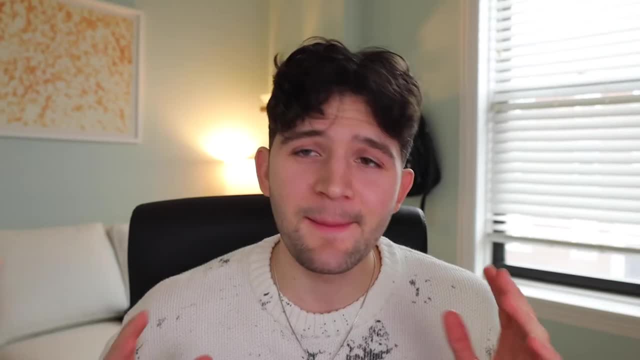 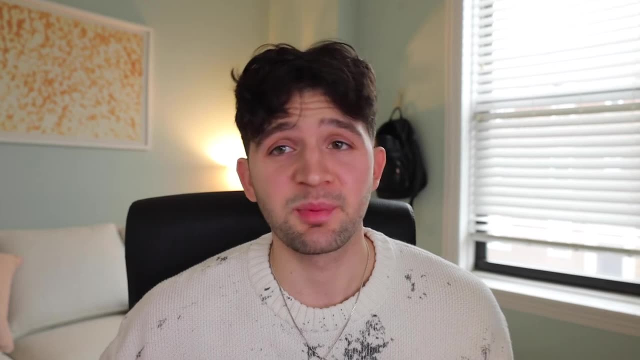 pretty much all day. you enjoy working with computers, you have a base understanding of how a computer works and you're looking for a challenging yet fulfilling job which honestly pays pretty well. That's. that's another good side note, And if you really want to make an impact on 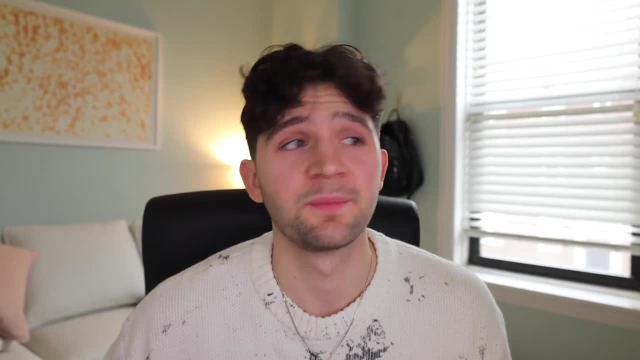 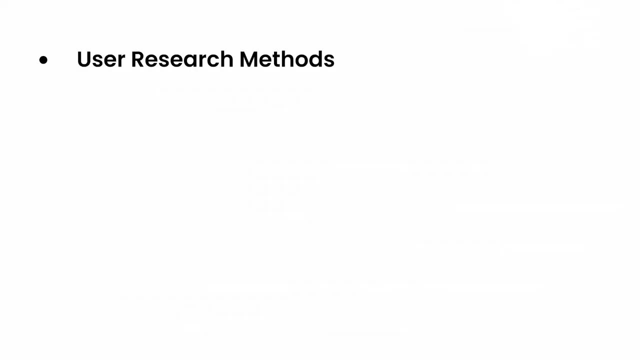 people's lives through technology, then this is the right major for you. So just to list off some of the classes that I've taken so far at DePaul University, studying HCI, I have completed user research methods, statistics and data analysis, website design and data analysis, And then I've 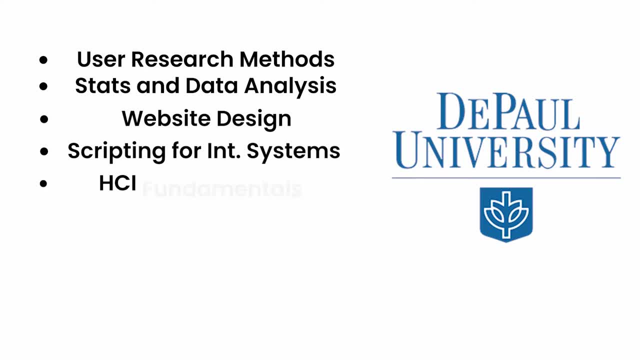 also done a lot of research on data analysis. So I've done a lot of research on data analysis, website design and data analysis. And then I've also done a lot of research on data analysis, website design, scripting for interactive systems, HCI fundamentals, global user research. 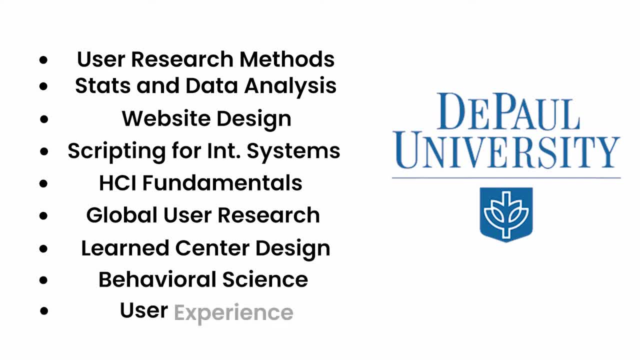 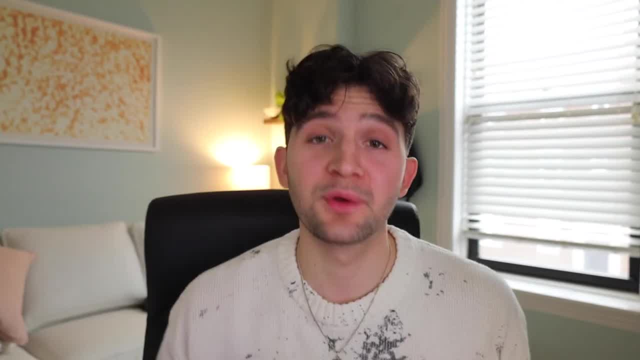 learned center design, behavioral science and user experience. Those are literally just a few classes that I've taken so far, But that kind of gives you a little bit of an idea of the classes that you will be taking. So the reason you guys are here: is it worth it getting an HCI master's? 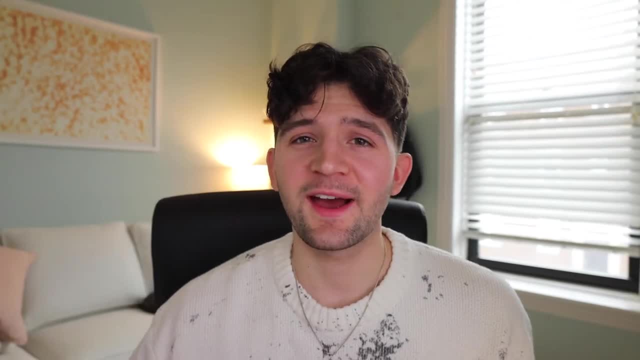 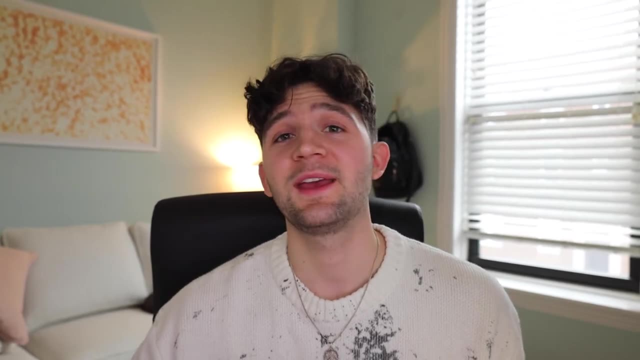 degree, I would say yes. However, I think this goes person to person. you should always be outweighing your costs, how much it is to go to whatever school that you have applied to, and if the value really outweighs how much you're paying And, fortunately, when it. 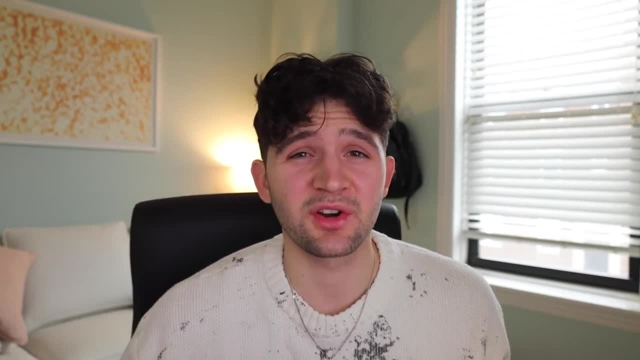 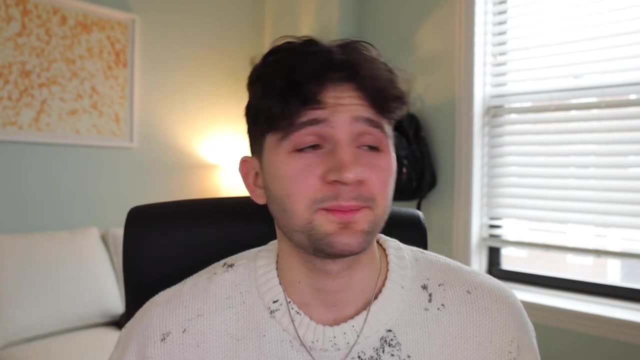 comes to HCI, I think the knowledge and, honestly, just project earnings that you get when in school far outweigh the cost that you pay. This is just me, but that's my opinion Now, since I'm actually working in the industry at the same time getting my master's degree. you may be asking: why are 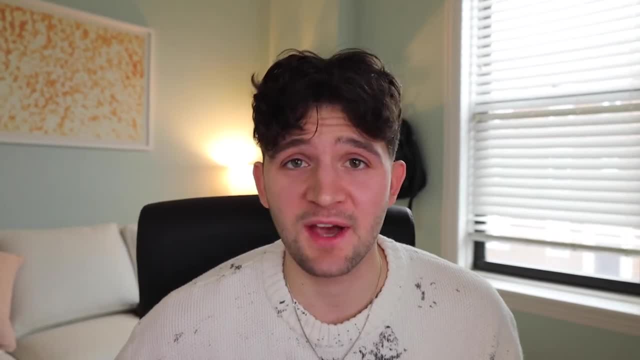 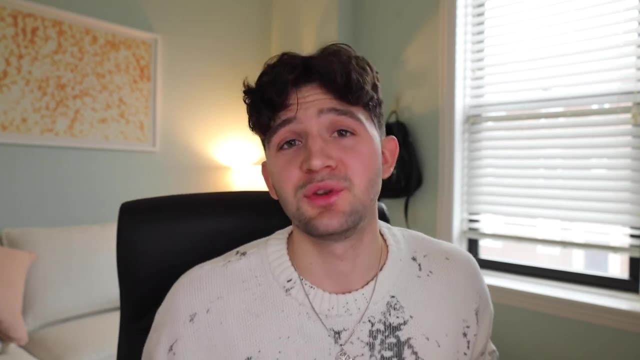 you doing that And honestly, it's just because I love learning about the topic And I think getting a master's degree in it just proves that I'm really passionate about it. It shows employers that I'm really wanting to do this for a living and it's something that really 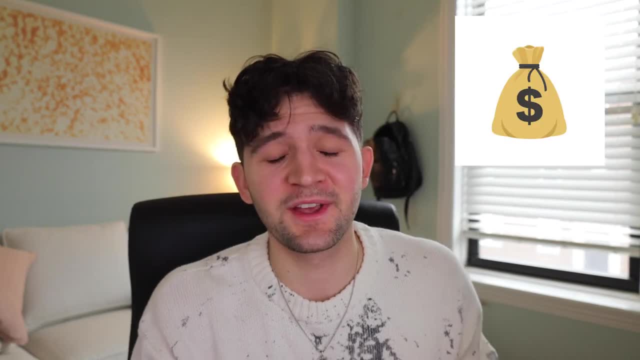 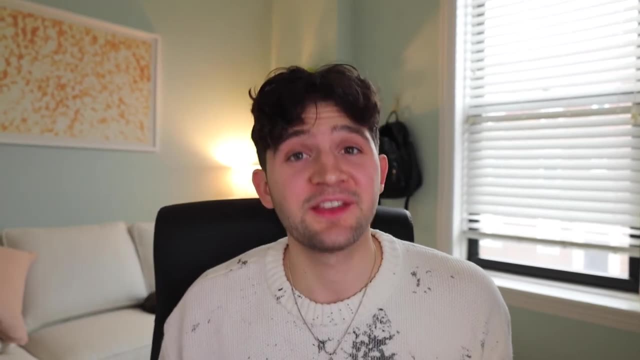 excites me. It's also worth noting that you get paid more when you have a master's degree in it. So yes, in the end, I do think it is worth it getting the degree. I think you'll enjoy the studies a lot and you will be challenged a lot. A lot of this is a lot of theory and idea seeking. 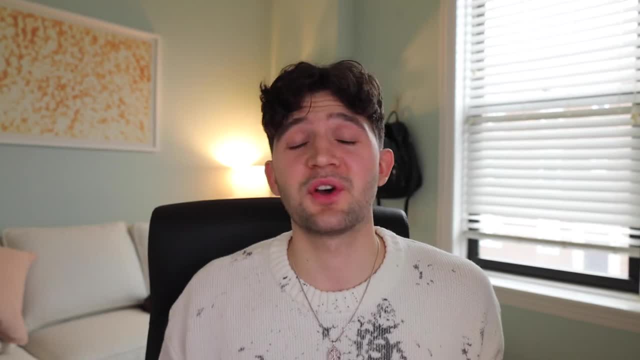 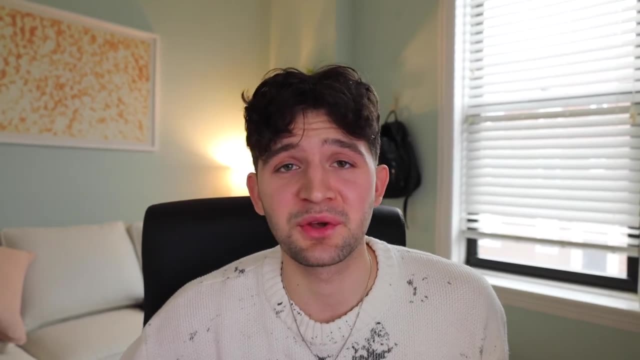 understanding statistics and data analysis. That is all really critical when doing user research And, honestly, some of it cannot be very fun. Like I said, there are so many careers that you can really go down And that alone, I think, is worth the HCI component. So one thing that I also want: 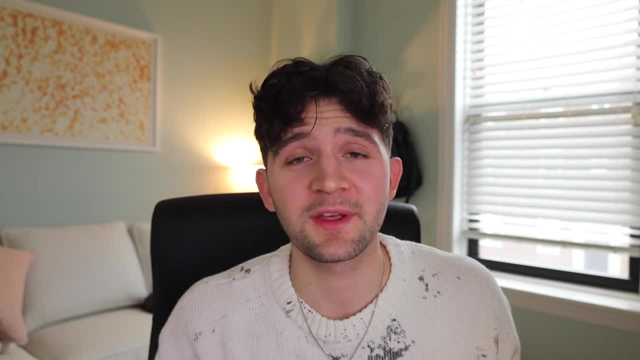 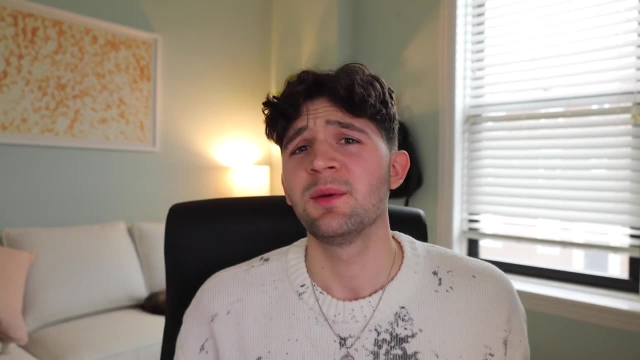 to note, because people ask me all the time is: will you have to code in this degree? And yes, you will. Only for a little bit, though. My introductory classes were a lot of coding, usually a lot of front end coding. I didn't really do a lot of like back end, but you will. 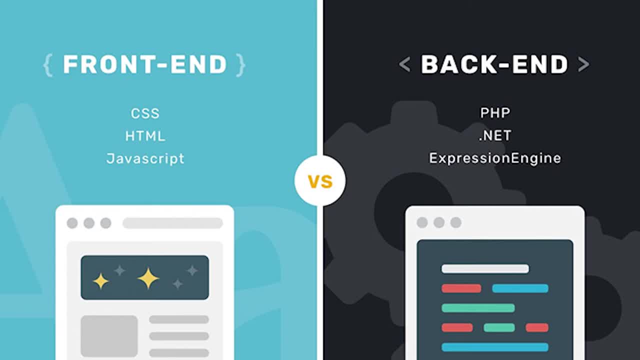 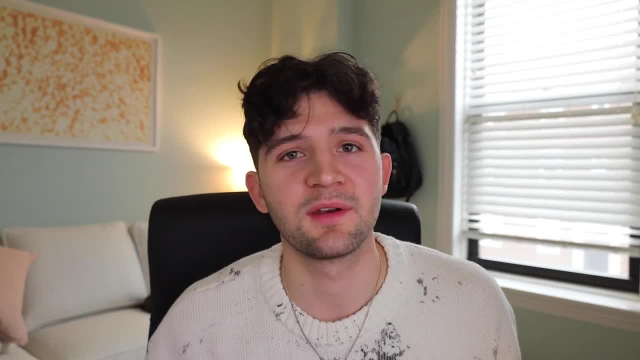 have to learn, like JavaScript, HTML, CSS, just the basics. You're not going to be like developing a super complex app, but you will be making interfaces, Making things that people can interact with. You'd be surprised how quickly you can catch on.